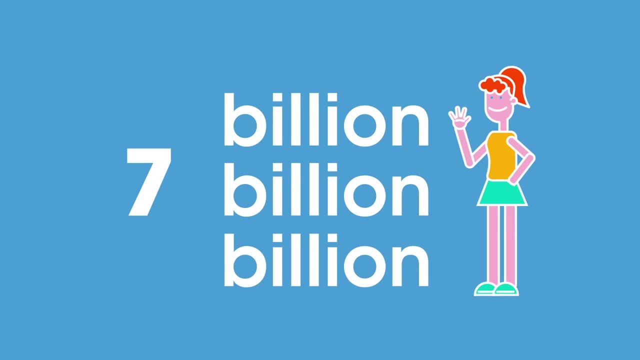 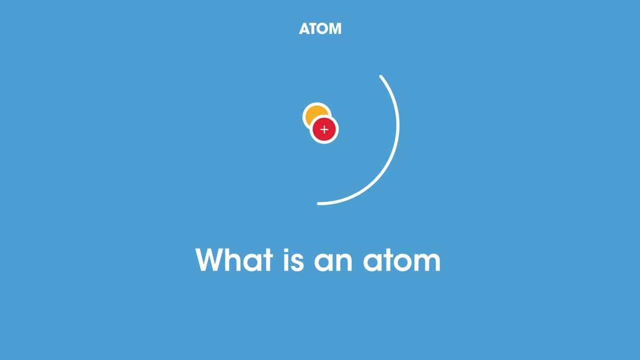 there are about 7 billion billion billion atoms in your body alone, which is 7 times 10 to the 27 atoms. But what is an atom? In this video we are going to look at what atoms are made of and the mass and size of atoms and the arrangement of electrons in an atom. Atoms may be tiny particles. 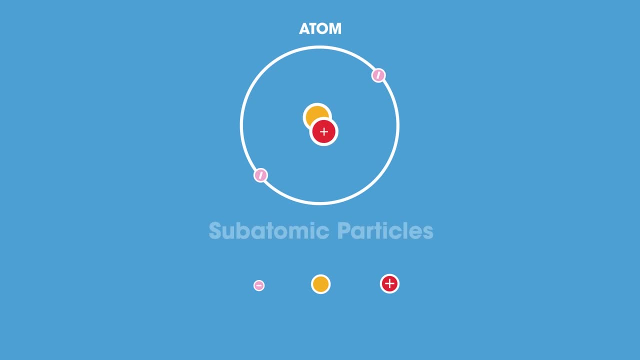 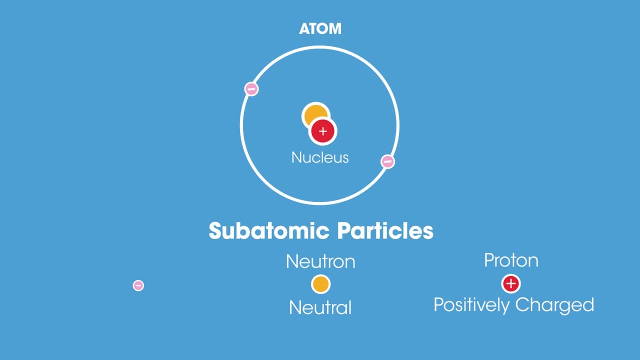 have no charge. This makes the nucleus overall positively charged. Much like how the Sun has planets orbiting it, the nucleus has electrons orbiting. Electrons have a negative charge. Because electrons are negatively charged and the nucleus is positively charged, they are electrostatically attracted to each other, Like how gravity ensures attraction between 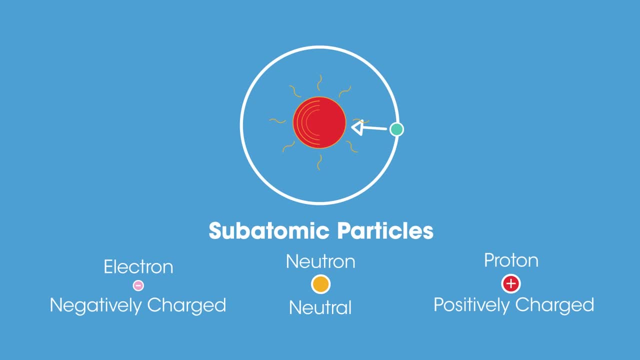 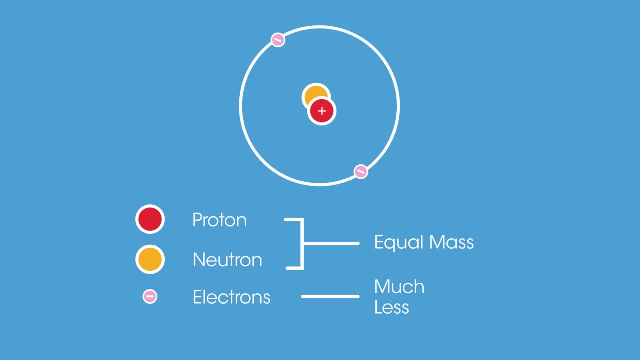 planets and the Sun. So that's the general structure of an atom. What about its mass and size? Protons and neutrons have the same mass, but electrons are so small they weigh almost nothing in comparison to protons and neutrons. In fact, they are around 2,000 times lighter As a 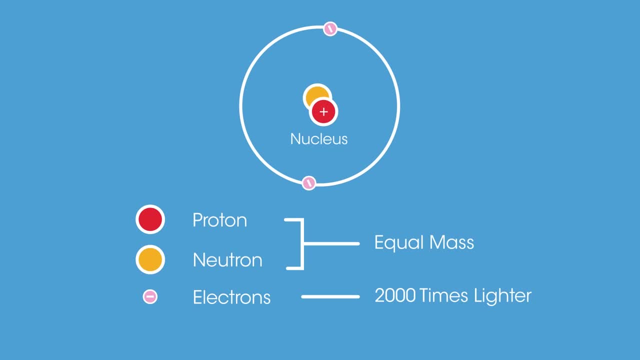 result, the mass of an electron is concentrated at its nucleus. So that's the mass of an atom. Let's talk about its size. One way to describe the size of an atom is its radius. The radius of an atom is the distance from its centre, where its nucleus is to the outermost. 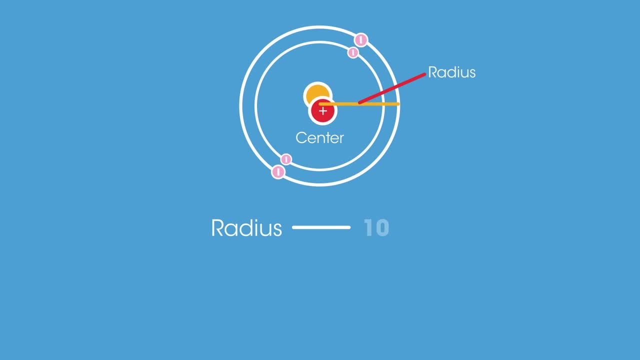 shell of electrons. The radius of an atom is typically 10 to the power of negative 10 meters, which is very small. So the majority of the mass of an atom is contained in its nucleus, But in terms of size, the nucleus is much smaller than the atom as a whole. In fact, electrons can 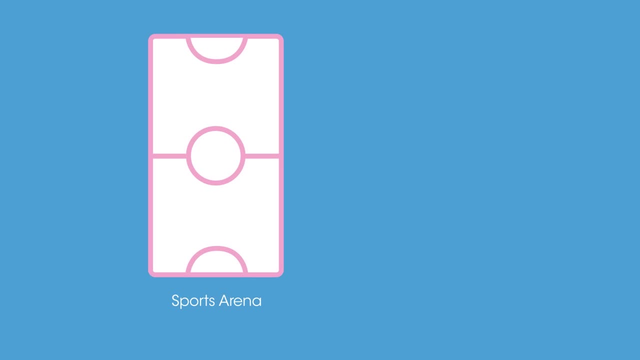 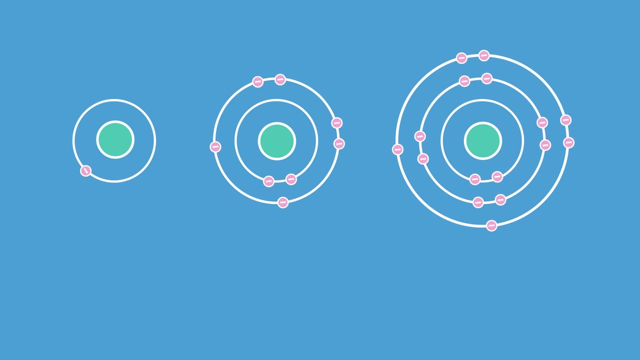 orbit really far away from the nucleus. If the atom was the size of a sports arena, the nucleus would be the size of a pea in the middle. Let's finish off by looking at the electrons in a little more detail. Negatively charged electrons orbit around the positive nucleus in specific.